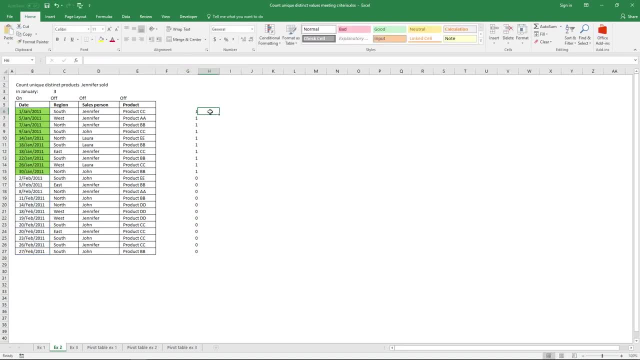 second, one logical expression and the question is: how many unique, distinct products are that did Jennifer sell in January and we have done the date criteria or condition and now I want to know if the dates are in January and the remaining dates are in January and the remaining dates are in February and it's forward. so I'm just 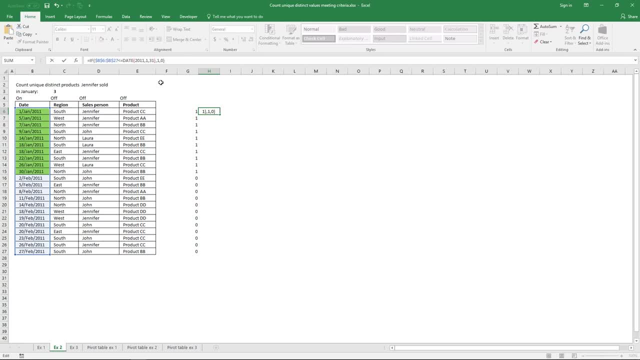 going to write a book? Yeah, so independ tackle here, right, and then I'm going to create an alternative API to this, which is a custom API to Jennifer, and then after that I will click change which equals Jennifer, and then I can properly open an nghĩ. and here I am. 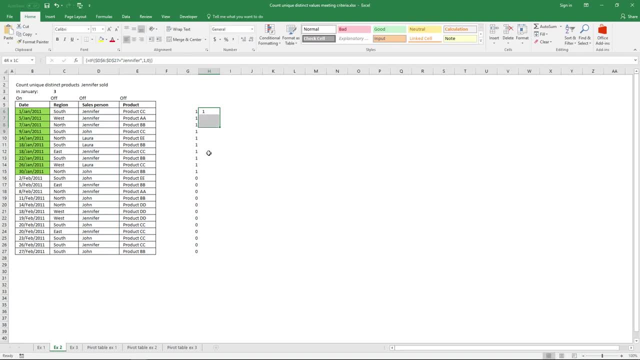 tôi đang t楽a, and the array here returns one if Jennifer is in this place is here, and zero if other name is here, and I made a conditional formatting formula to highlight those values. so if we combine these logical expressions, you can see. 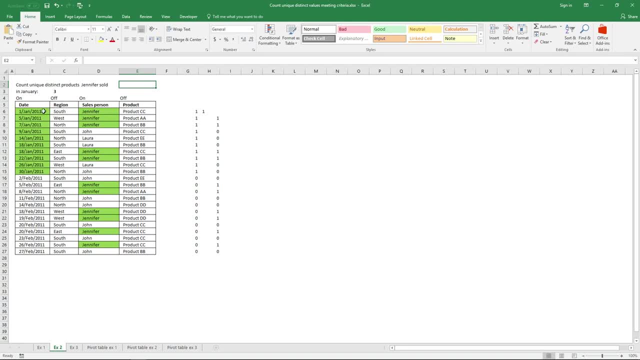 that if both January and Jennifer is here, these values here must be counted. and to do that I'm going to combine the logical expressions- and here is the first logical expression- and I'm going to multiply them. so I need a beginning and ending parenthesis around the first logical expression and 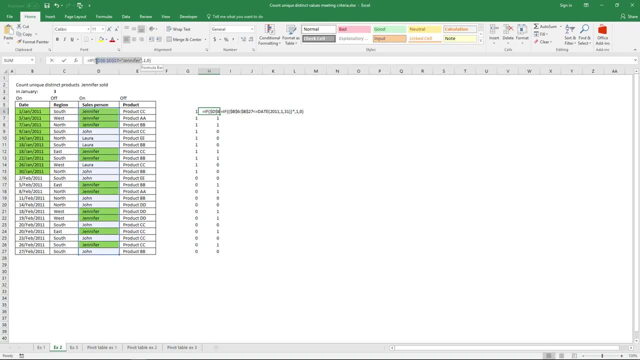 the second one is this one copy that: beginning parenthesis, ending parenthesis and now the array looks like this: here and here, and here they are. so the count ifs function shall count these products here. so the second part of the formula uses a count ifs function to count products. 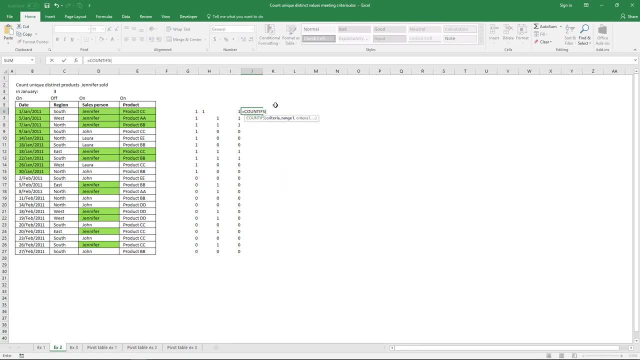 equal sign, count, ifs, and- and I'm going to use a cell range both in the first argument and in the second moment like this: and now this count is function counts, the plus value in this cell range here, how many times it exists in this cell range, and it returns eight from this value here. 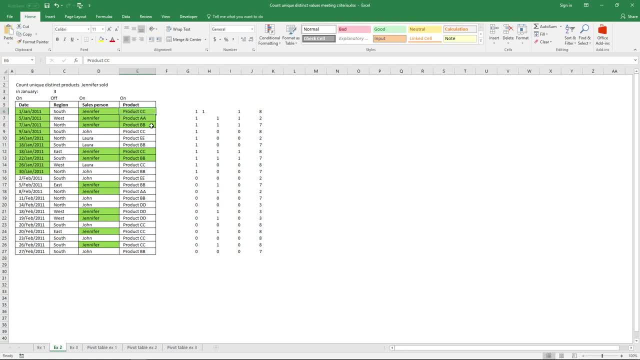 so there must be eight of this of this value here, one, two, three, four, five, six, seven and eight. and if you divide this array here with one, one divide like this, one divided the values. now, if I sum these values here they return unique, distinct, the count of unique, distinct values in this cell range here. 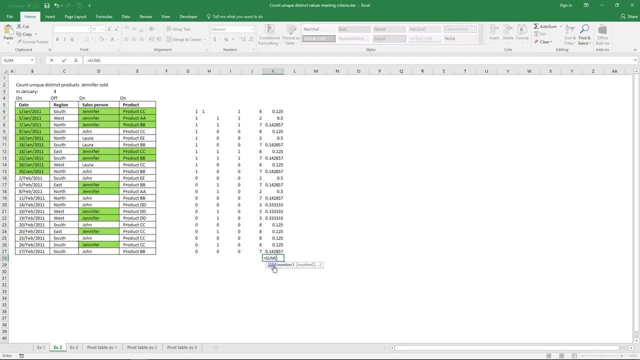 so there are five different products in this cell range here: one, two, three, four and five. so that seems to be right. and if we add the values for these products here, sum, and these two cell ranges here, you will see that they. they don't match up. the. this should be a, an in a whole number, no decimals and. 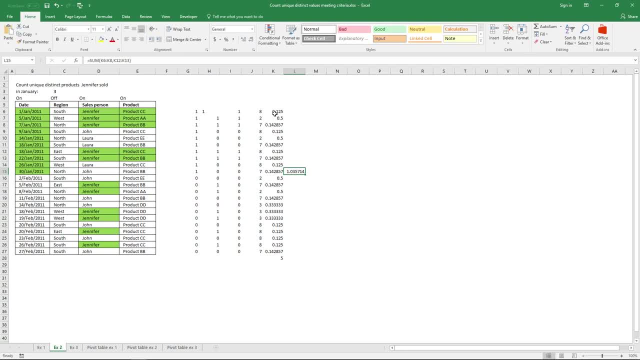 so this count here I can't use this one, so I need to use more conditions in the countries function for this to be right. to do that, I simply copy this OK and add more criteria here and one criteria is the Jennifer and the criteria range is this range here and I also need to make to have the dates in. 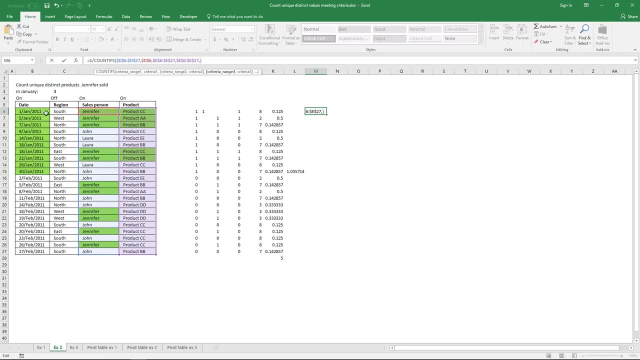 January, and to do that I need to select this cell range and this is criteria range 3, and then the logical operators and present and the date. 2011 and 31 extend this and enter it as an array formula and I'm going to sum these values to see if they match up. they are right and this: 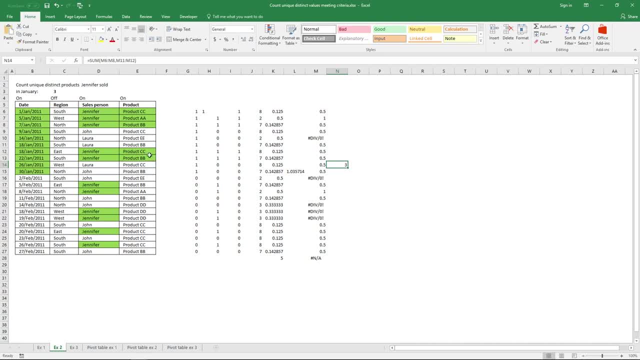 tells me that there are three, and this tells me that there are three unique, distinct products in this event. unique distinct products in this event. unique distinct products in this event, here and here, and here's one. here is one. here and here's one. here is one, here is one. 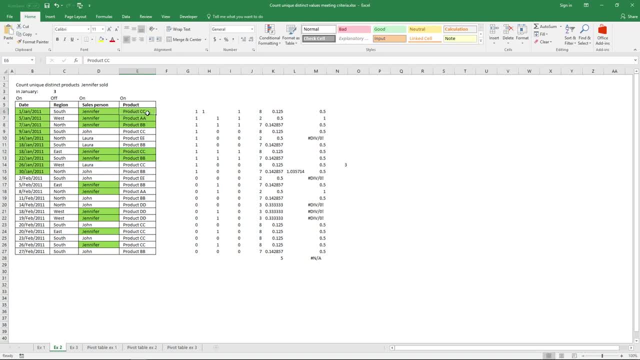 here, and here is one, here is one, and here is one, and this is a duplicate of. and here is one and this is a duplicate of. and here is one, and this is a duplicate of this, and this is also a duplicate. so this and this is also a duplicate, so 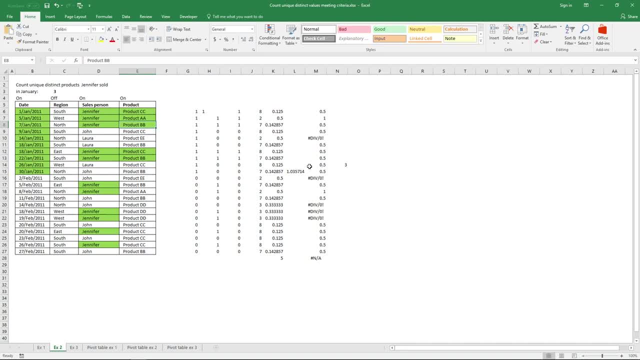 this and this is also a duplicate. so there are three unique, distinct values. there are three unique distinct values. there are three unique, distinct values, and now I'm going to combine the if, and now I'm going to combine the if, and now I'm going to combine the if function with the count ifs function. 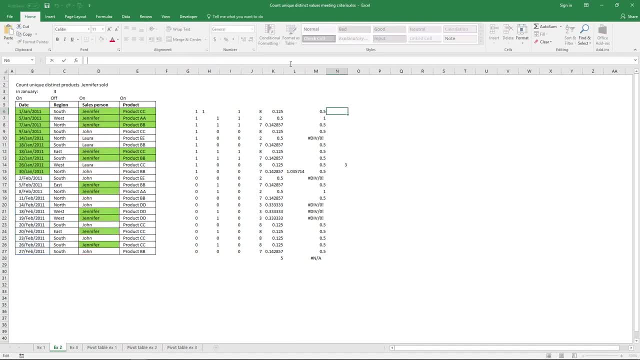 function with the count ifs function, function with the count ifs function, And the countifs function is here, And if these logical expressions return true, I want the countifs array, And if they return false, I want nothing or zero. And now I can sum the array.